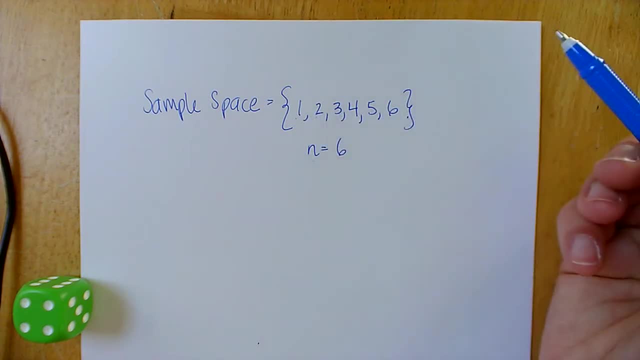 here, or the number of outcomes. remember, we like to use the same word to represent different words, to represent the same concept: One, two, three, four, five, six, A total of six. Okay, let's go on and find some probabilities. 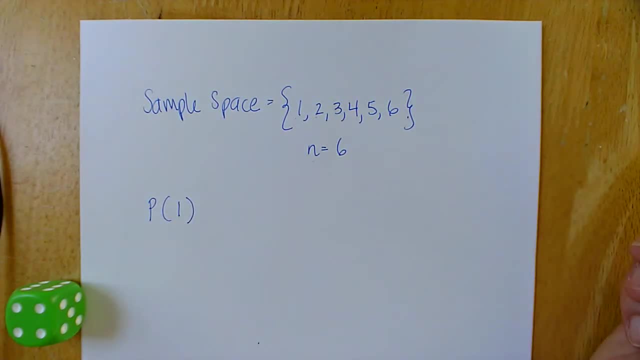 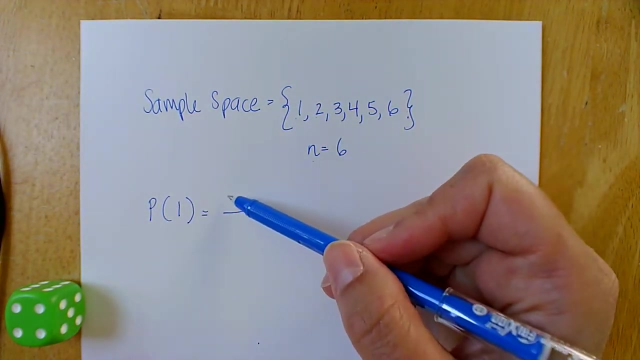 So if we want to find the probability of the rolling, the event of rolling number one- little tongue twister there- if we want to find the probability of rolling a one which our event is rolling a one, we have to use our rule number four, which was how many ones on the die divided by the 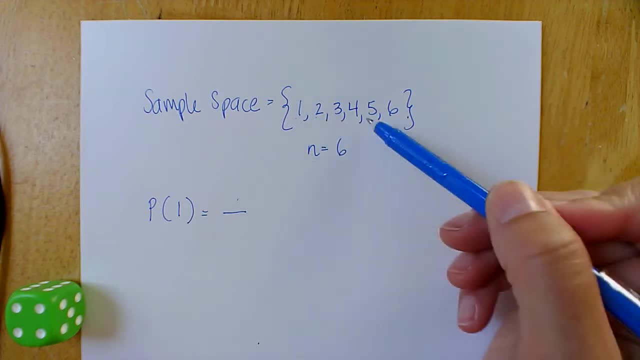 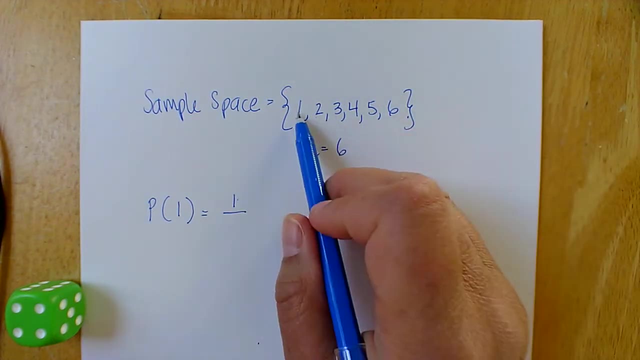 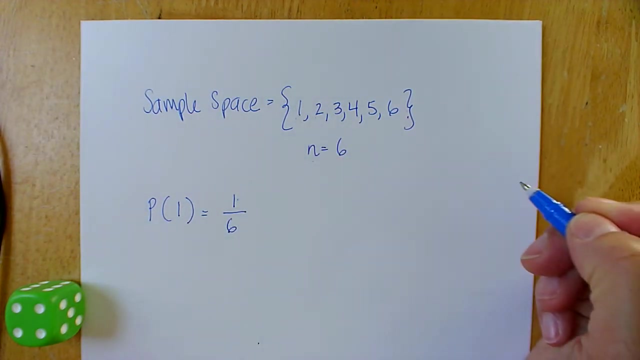 total number of six Samples, or the total number of numbers which is our sample space. So, how many numbers? how many ones are there on our die? There was only one, and that only came up once. Okay, how many total numbers do we have? We have six, So we have a one out of six chance of rolling a one. We can reduce this and 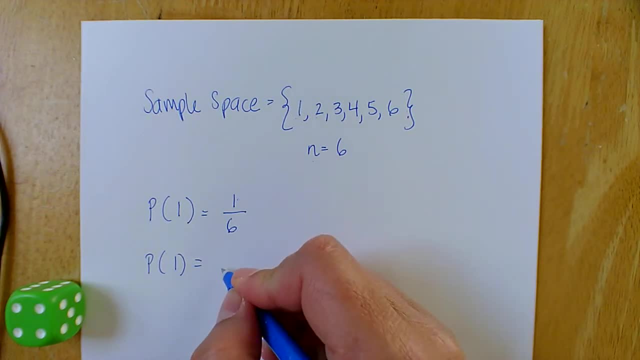 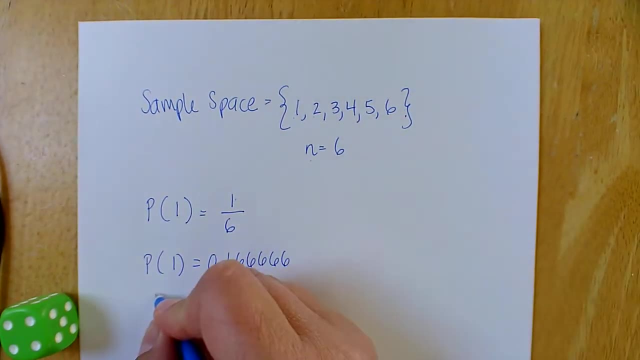 when we divide it out, actually we can't reduce it, we can divide it out. When we divide it out, we get 0.166666 repeating. Okay. so if you would like to, you can round that to 0.17.. Absolutely fine If you want to change it. 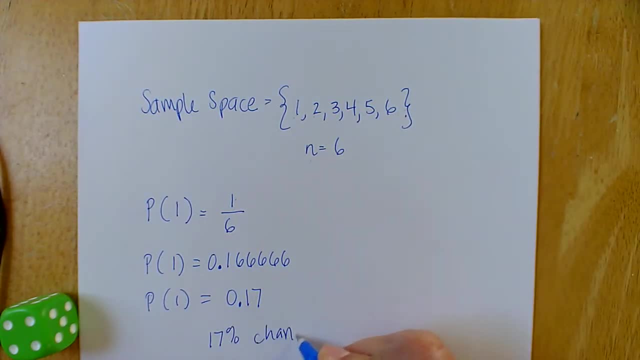 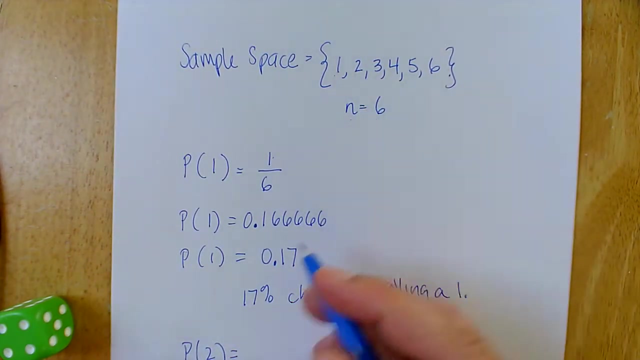 into a percent chance. we have a 17 percent chance of rolling a one. Okay, well, let's do all of the others quick. Probability of rolling a two. Well, there's only one, two in our sample space. so there's only one, two out of. 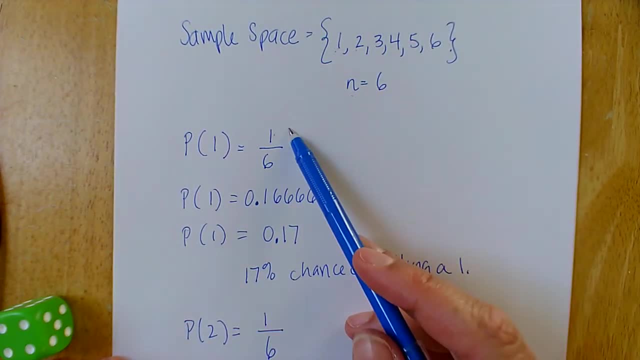 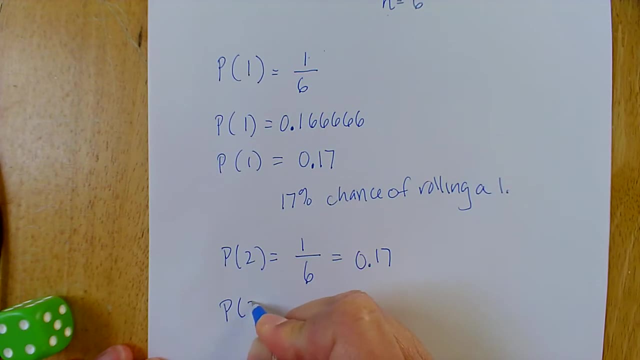 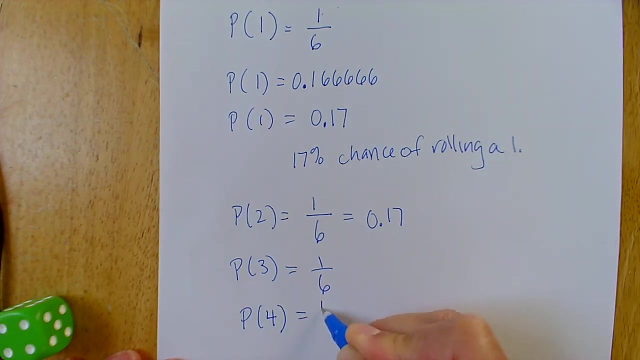 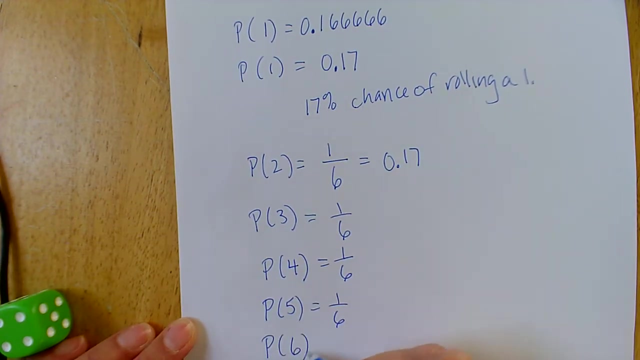 six total, So one out of six, Same exact as our probability of rolling a one, which is 0.17.. Well, probability of rolling a three: again one out of six. There's only one out of six total. Probability of a four: again one out of six. Probability of five: again one out of six. And, lastly, probability. 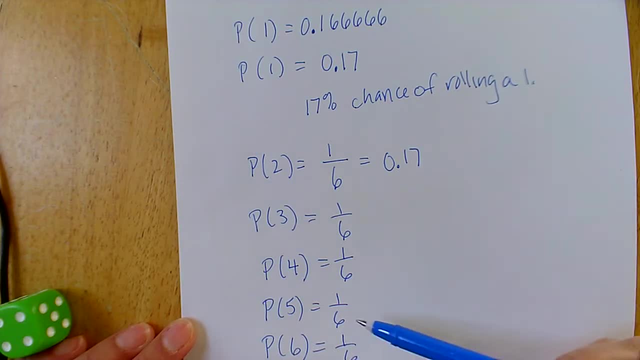 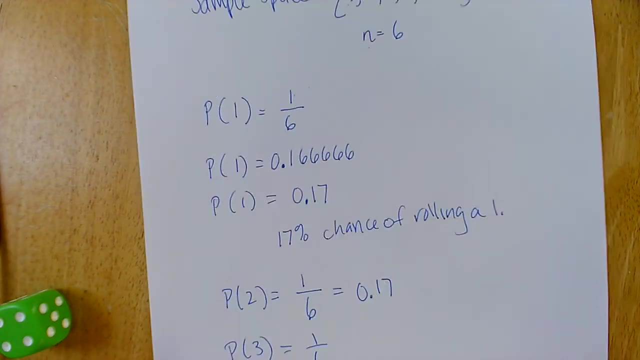 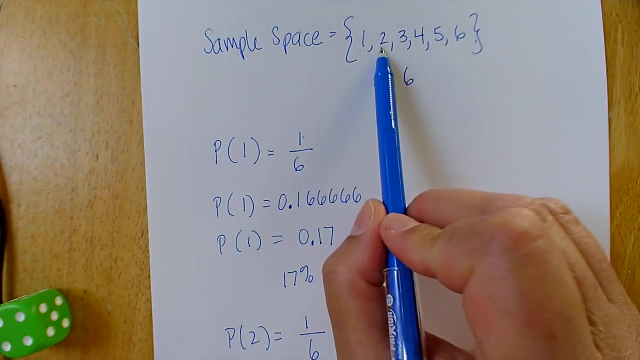 of rolling a six, one out of six. So notice, each one of these has the same chance of being rolled, And that's what it meant by a fair die. We don't have. it's not weighted, which means that the two isn't going to come up more often. The two is going to be rolled. 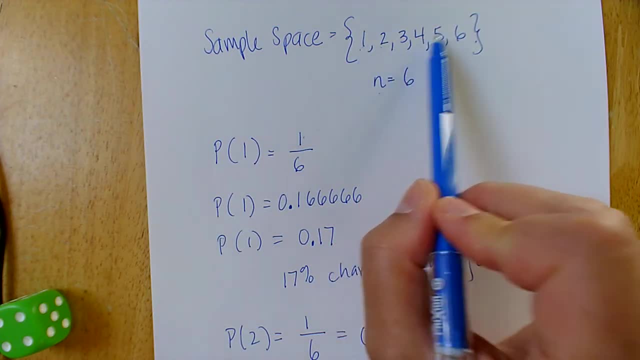 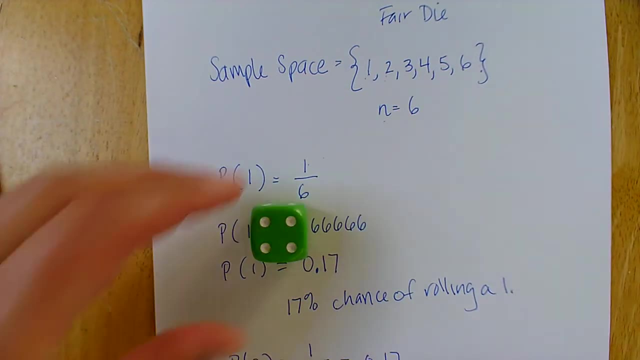 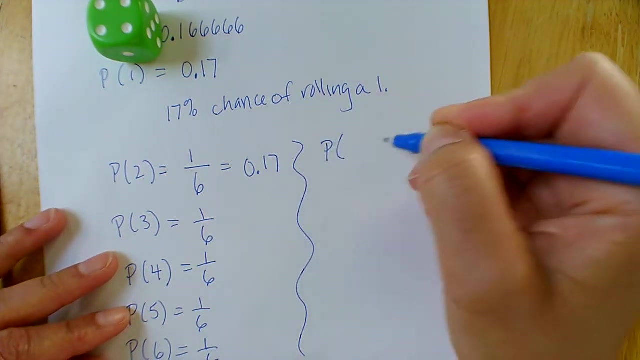 as many, we have the same probability of the two being rolled as any other number. So this is a fair die. Okay, let's look at some other probabilities. I'm going to make a little break right here. Let's find the probability of rolling a one or a two. Okay, so remember that's the outcomes divided by. 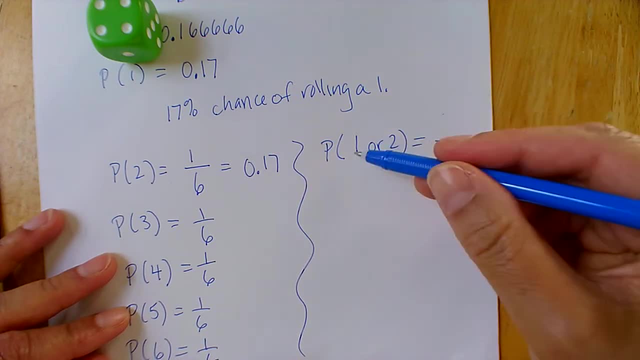 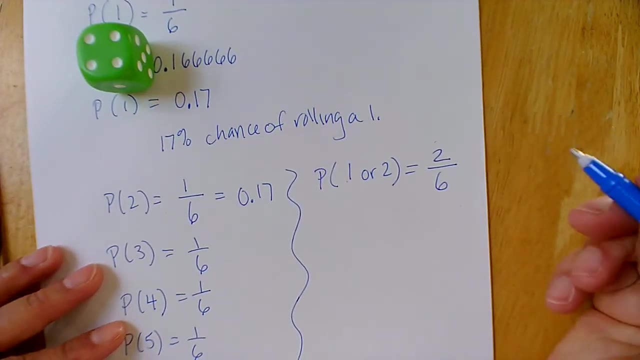 the total number. We have six in our sample space. How many one? how many two? So we have one, two, That's it. So we have a two out of six chance of rolling a one or two. We can divide that out to. 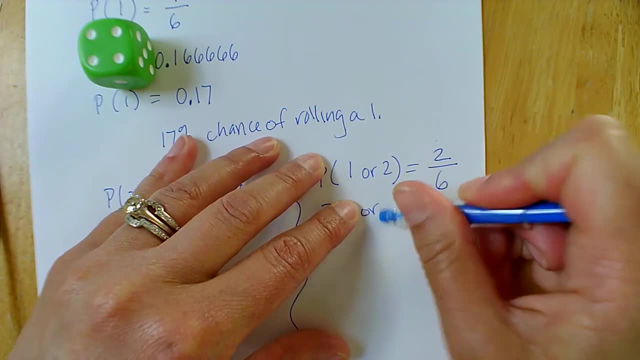 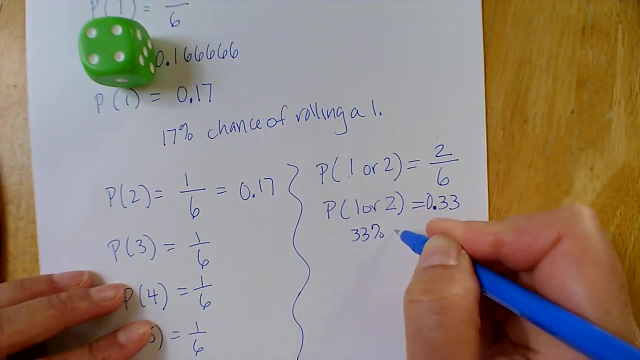 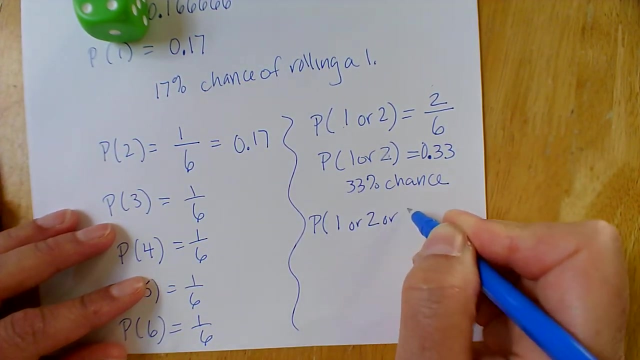 be point three. oops, I was saying point three. We can divide that out to being zero. point three, three or a 33% chance, All right, how about the probability of a one or a two or a five? 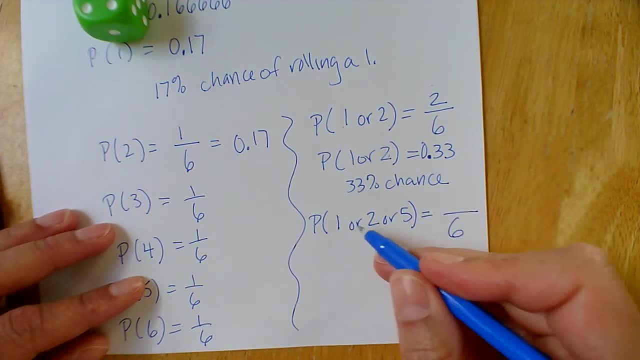 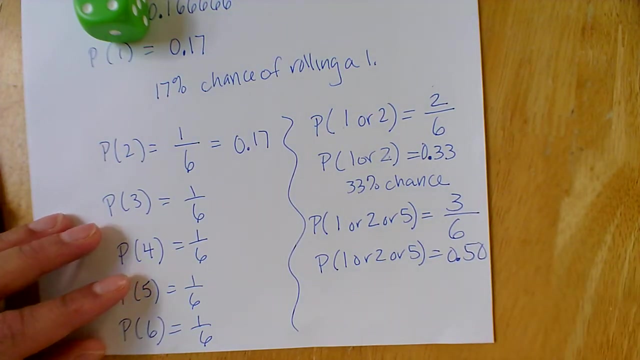 Well, we know, in our sample space there's six numbers and one, two, three. there's three outcomes, So that's a three out of six, Three, one, two, three out of six total. So the probability of a one or a two or a five is zero, point five, zero Okay. 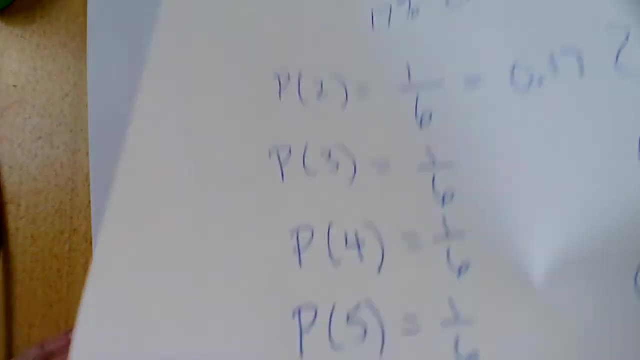 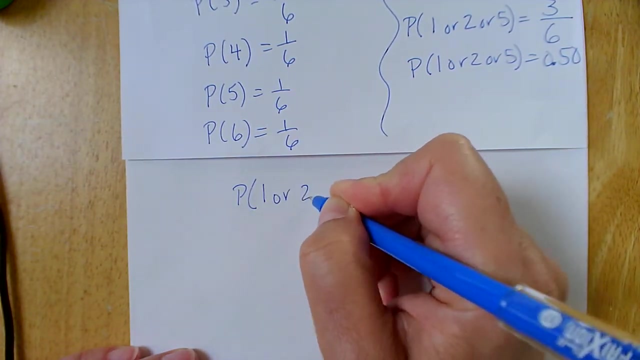 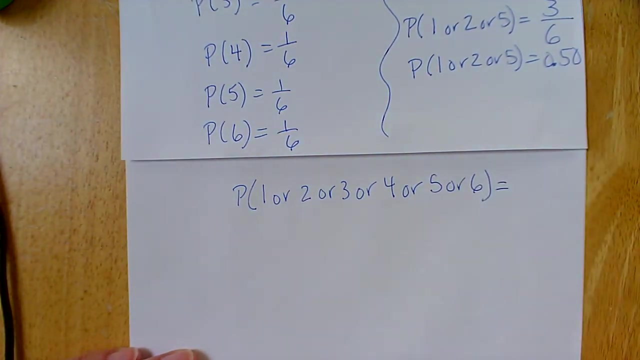 let me throw this one at you. How about the probability of a one or a two or a three or a four or a five or a six? Let's say I was going to give you $1,000, 1,000 bucks if you rolled a one or a. 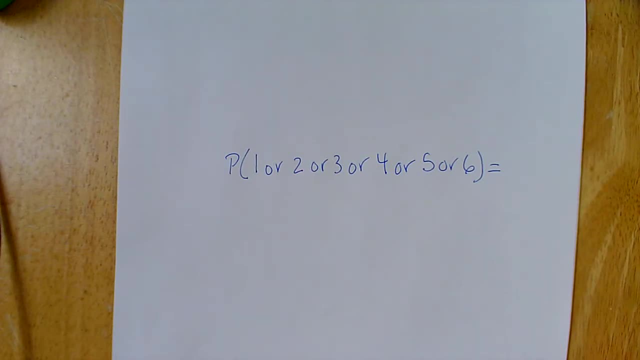 two or a three or a four or a five or a six. Would you take it? Oh, I would take that bet, Heck. yeah, because we know there are six outcomes. Well, I have here's outcome: one, two, three, four, five, six. 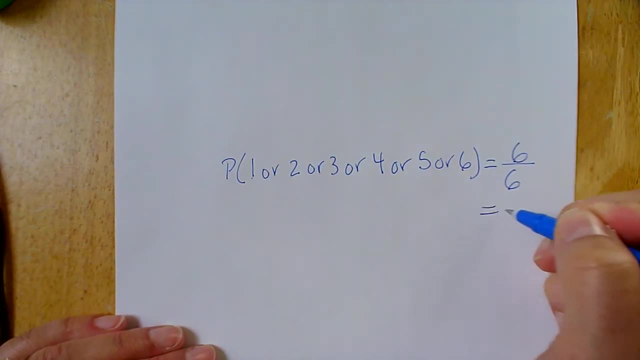 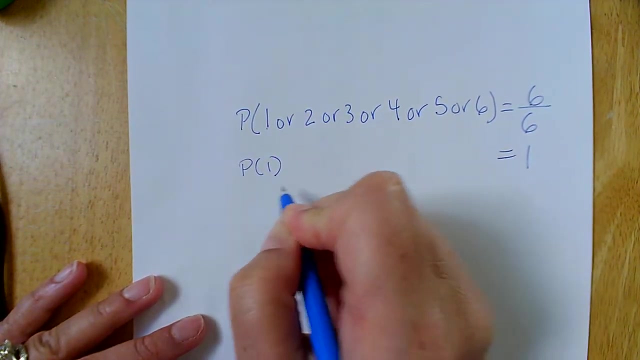 So we have a six out of six chance. That is a probability of one. We could have also done it like this: We know the probability of a one is one out of six. We know the probability of a two is one out of six. 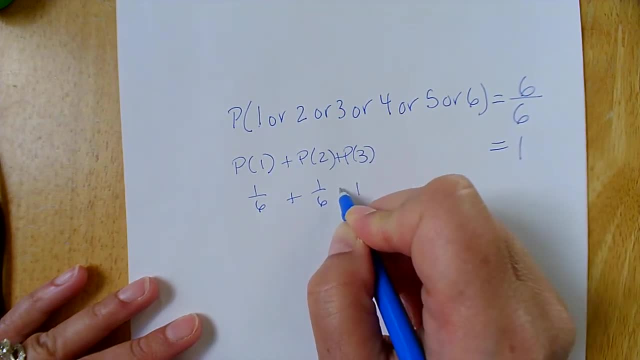 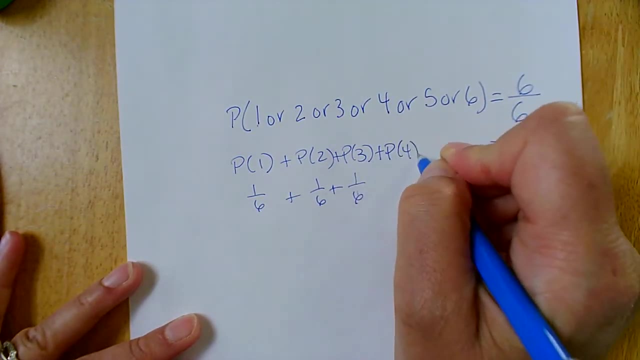 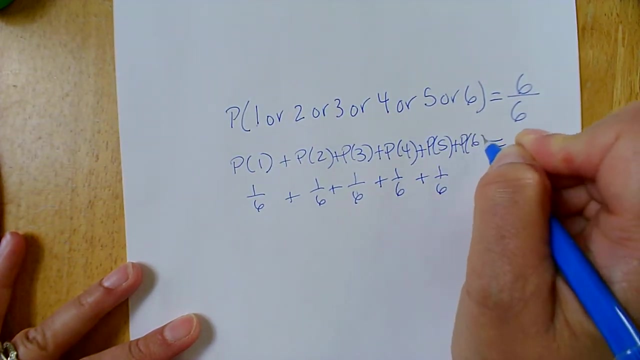 We know the probability of a three is one out of six. We know the probability of a four is one out of six. Probability of a five: one out of six, And the probability of a six one out of six. What do those add up to? 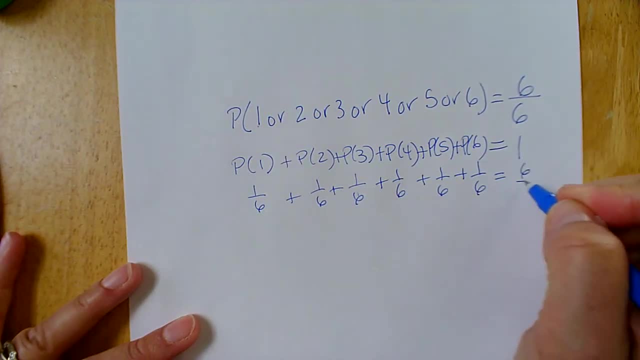 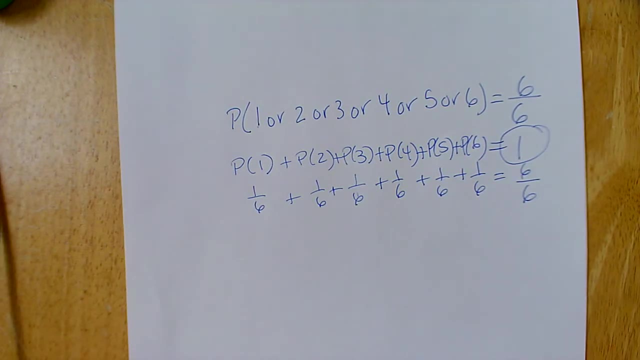 One, two, three, four, five, six, Six out of six, which gives us a probability of one. So if somebody says I have a six-sided die and if a one, two, three, four, five whirr. 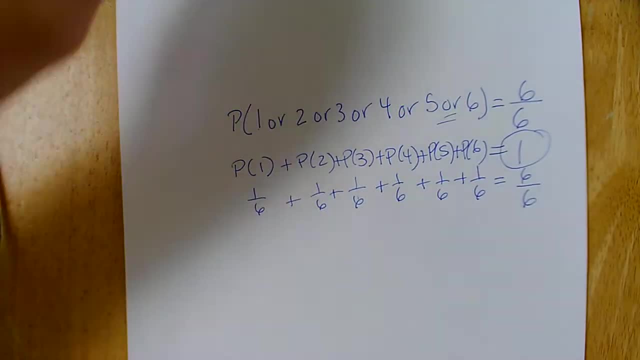 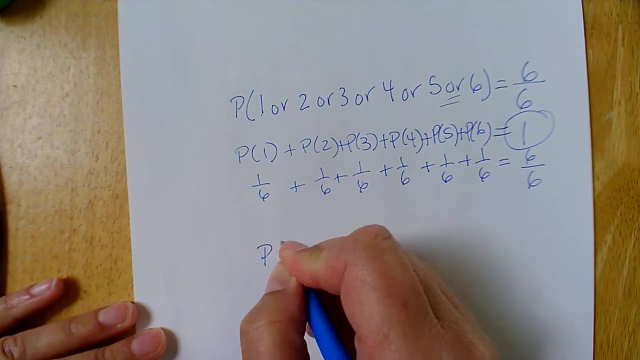 six comes up, you win. Take that bat, Okay. well, let's see What's the last one. Ooh, this one right here. Probability of a one and a two. Now remember we have a die, okay. 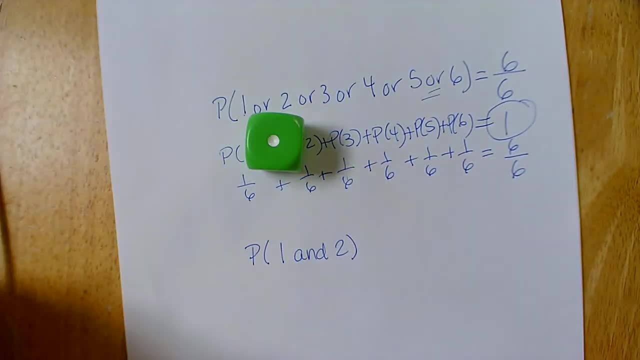 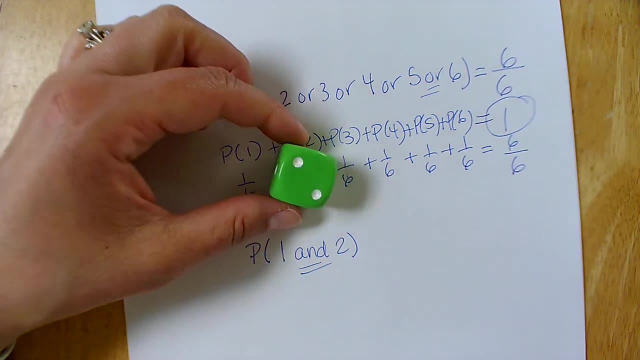 So we can get a four or we can get a one. We can get a one or we can get a two. I want a one and a two at the same time. You can't do a one and a two at the same time. 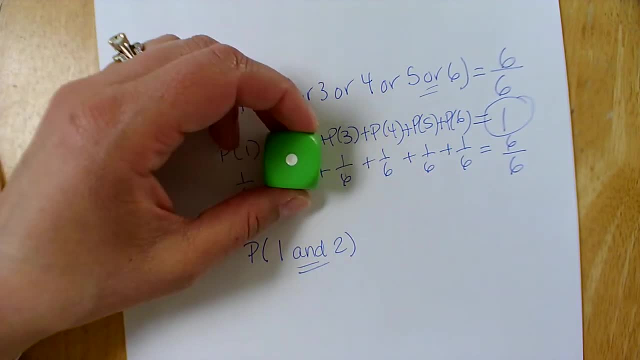 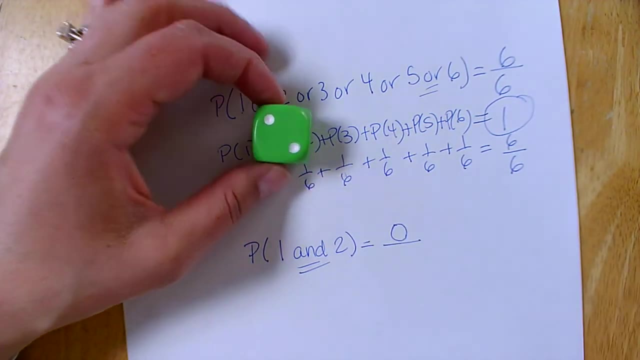 The die just doesn't fall like that. We have a one side, we have a two side, and that's it. So there's no sides that have a one and a two on this dice. There's no sides that have that using this dice right here. 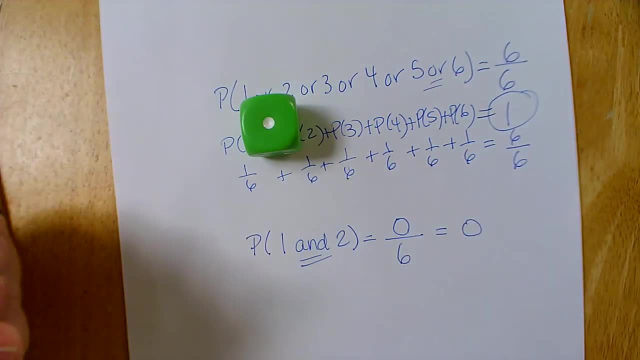 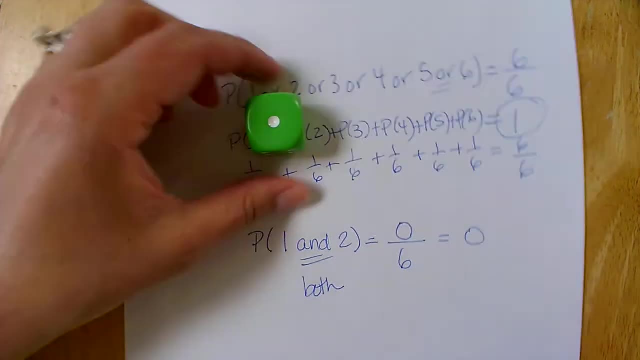 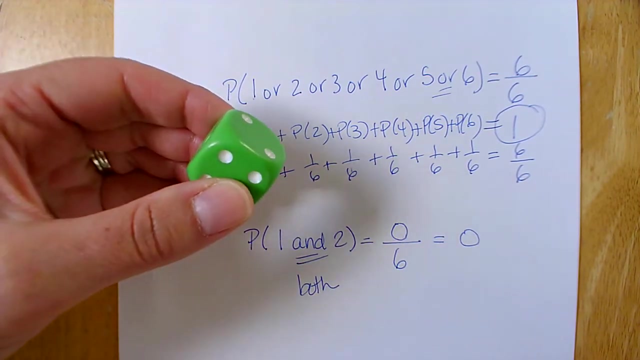 We have six possibilities. That gives us a probability of zero. So if somebody asks you to take that bat, don't take that bat. Don't take the both bat, especially when you're using a die. This has been finding probabilities using a six-sided fair die. 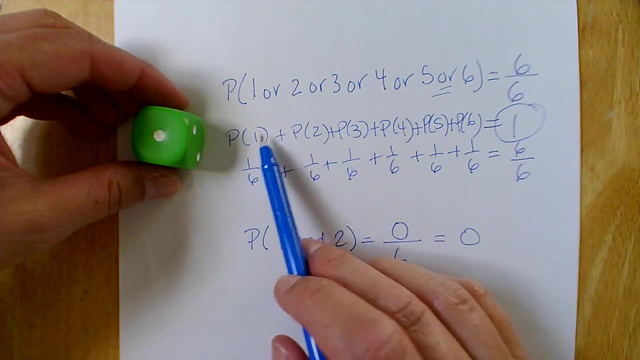 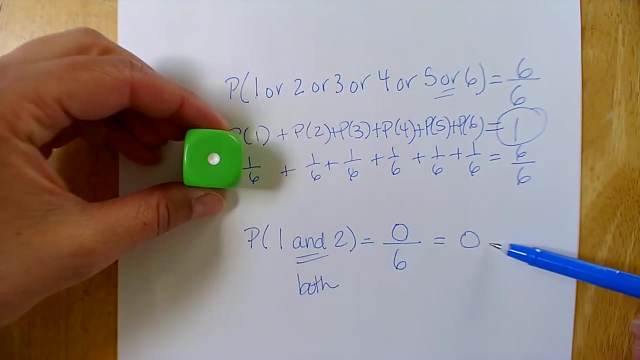 Adding them up. as you can see, if we add up the probabilities of all the numbers in our sample space, we get one. If we try to find both, we just don't have that on here. That's a probability of zero. 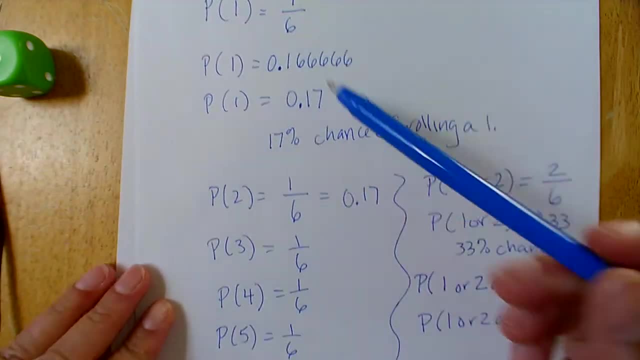 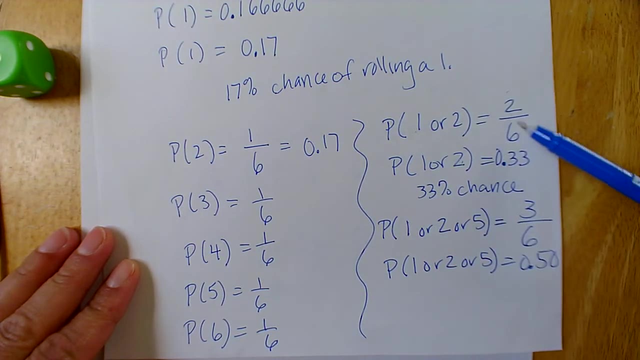 And we also found the individual probabilities one through six, And then look to see what happens if we have or or or, And we found that we can simply add those up as well. This has been Probability rolling with a fair die. Hope it helps. Thanks.